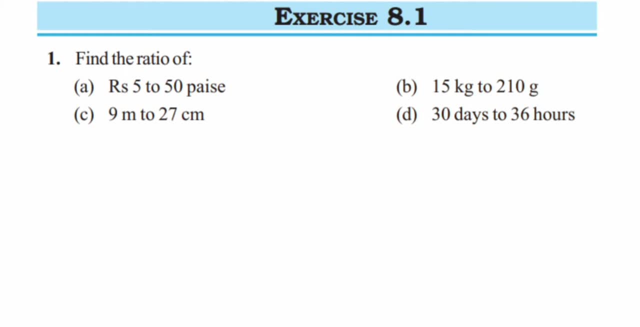 here is: whenever we are converting or whenever we are writing the ratio, we have to make sure that the units are same. So if you observe here in the first question, that is A, we have 5 rupees and 50 paise. So rupees and paise are two different units We have to convert. 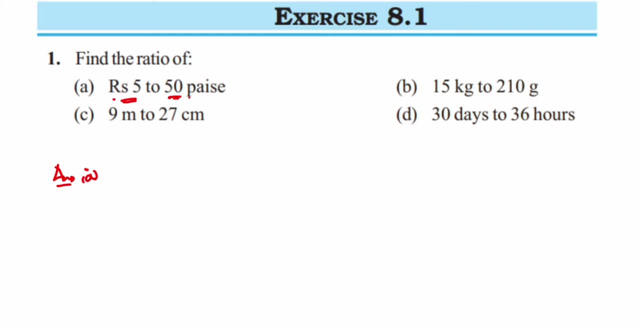 them into same unit. So what I am going to do here is we can convert paise into rupees or rupees into paise. In both the cases the answer will be a bit different. If you are converting rupees into paise, the ratio will be different. If you are converting paise, 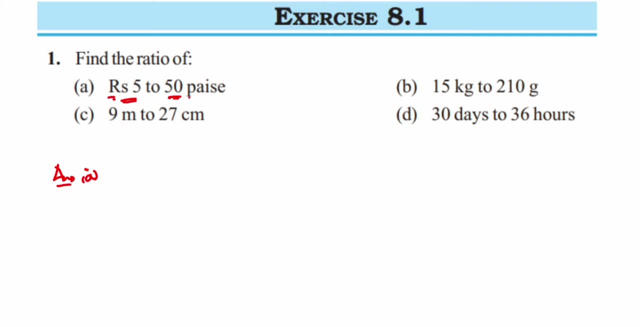 into rupees, the ratio will be again different. Here I am converting rupees into paise. We know that 1 rupees is equal to 100 paise, So we are going to convert this. We get 5 rupees, or rupees. 5 is equal to 500 paise, Just multiply. 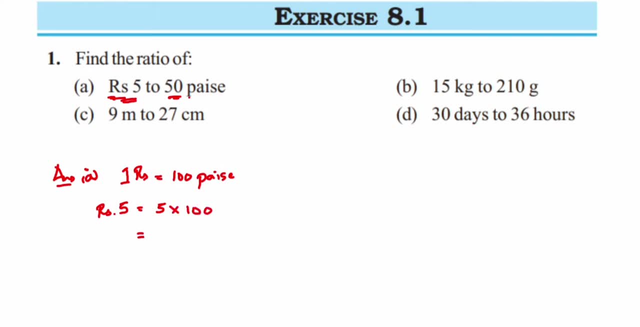 with 5. 5 into 100, which will be equal to 500 paise. Now we got both into paise. Now we are going to find out the ratio. So ratio of rupees 5 and 50 paise will be equal to, instead of 5 rupees. I am going 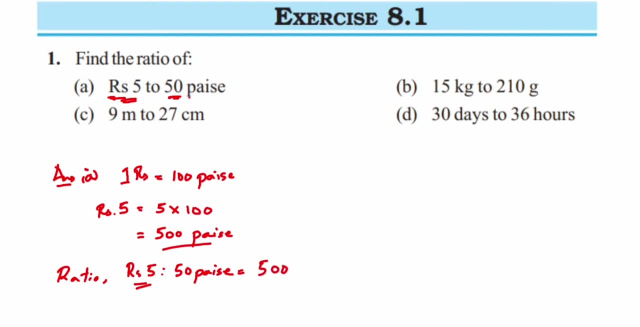 to write down: 500 paise. So 500 is 250.. Remember, whenever you are writing down the ratios, we don't mention the units here. So here it will be: 500 is 250.. Now we can reduce this further. 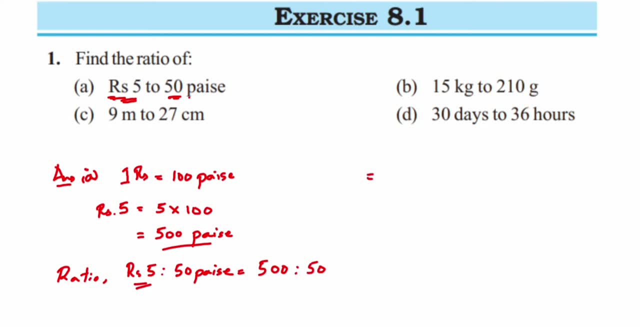 So this ratio, ishistory, So 5 over 50, I am going to write it down. In case we want to write down 500 paise, we can write the total ratio here. So 500 by 50 is called parcelation. 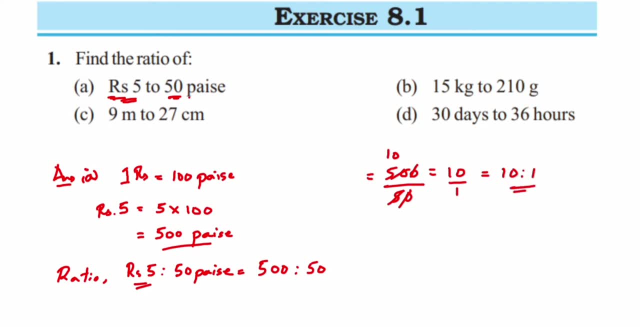 So I am writing down parcelation So we can write this as 10�-1.. the ratio for the 1st question is 10a to 1. into grams here, and then we're going to find out the ratios. okay, so for the second one, 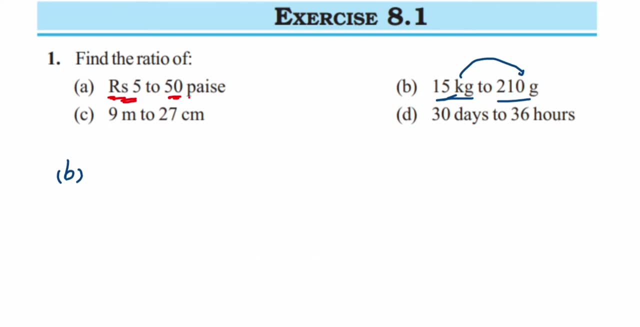 so we have 15 kg, right? so we know that 1 kg is equal to 1000 grams, right? so in that case, 15 kg will be equal to 15 000 grams. that is, 15 into 1000, 15 000 grams. now we're going to find out. 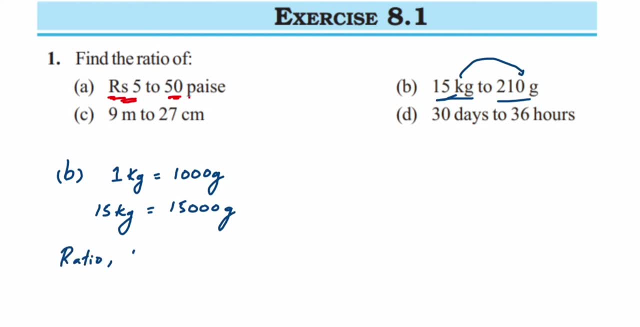 the ratio. so ratio of 15 kg to your is to 210 grams will be equal to: instead of 15 kg, i'm going to write down 15 000 is to 210. now again, we're going to reduce this. make sure that whenever you're writing down the ratio they should be reducible form. so for that again, i'm going to. 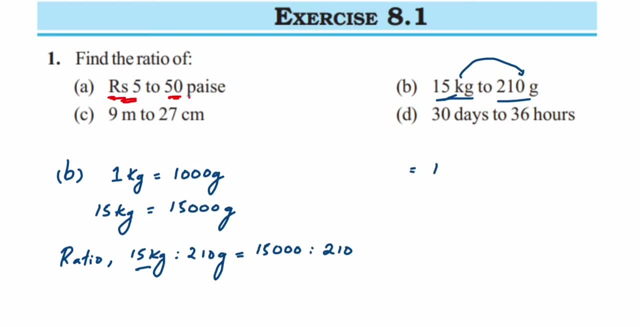 just perform a cancellation here. so this is 15 000. you can just do a cancellation here itself. like this, you can cancel. i'll just convert this into a fractional form and again i'm going to cancel it. so upon 210. see, here i'm converting ratio into: 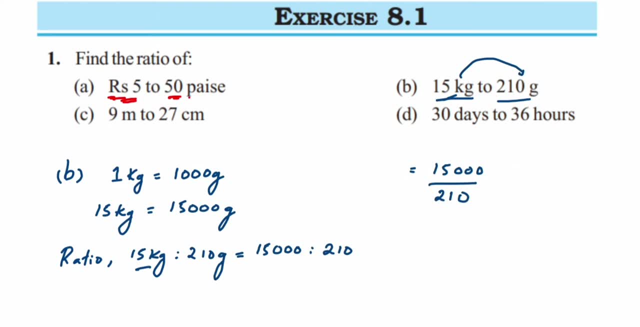 a fractional form and again i'm doing cancellation. you can avoid this and you can cancel here itself, so i'm going to cancel the zero. cancel this in three table. three sevens are 21 and then three fives are 15. two zeros will be here again. we cannot cancel this further. 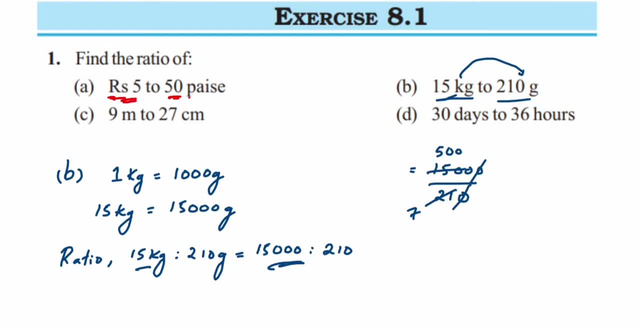 so because seven and five hundred seven is a prime number, we cannot cancel this further. so this will be 500 upon seven. so the ratio will be 500 is to seven. that's it now. the next question is we have to convert nine meters, so the ratio is nine meter to 27 centimeter. so again we're going. 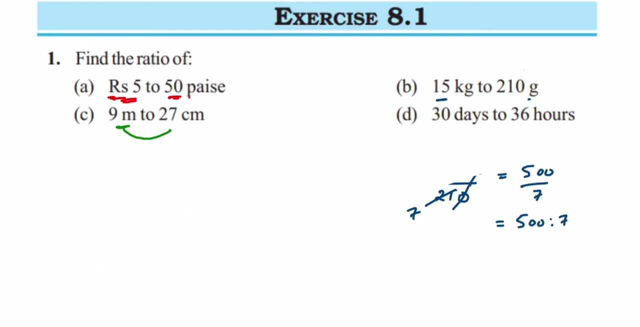 to convert meters into centimeter and again just reduce into the lowest form. so for the c problem, we are going to write down that one meter is equal to 100 centimeter. in that case, nine meter will be equal to 9 into 100, which is equal to 900 centimeter. now we're going to write down the ratio.